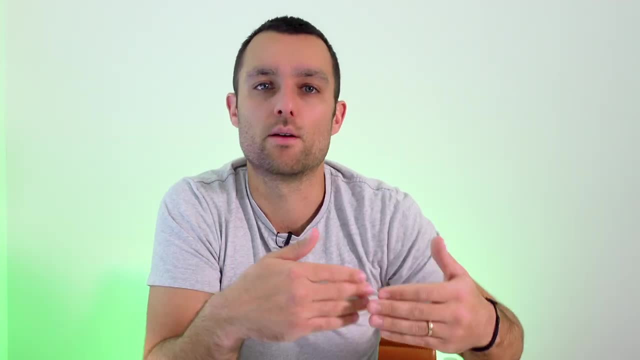 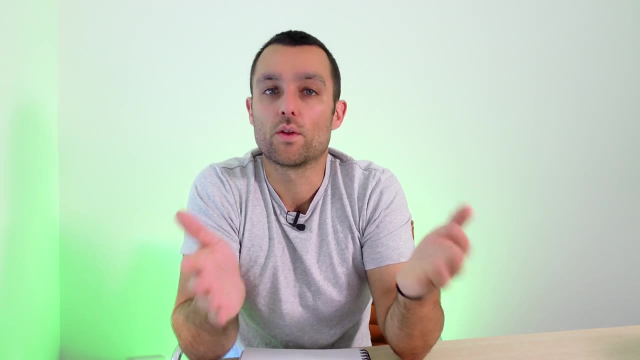 and with my clients. I always tell them I'm like it's better off that you just try and beat your own numbers, set your own baseline and try and beat your own numbers, Because a lot of these averages can often be not that good And I think is you're not being. 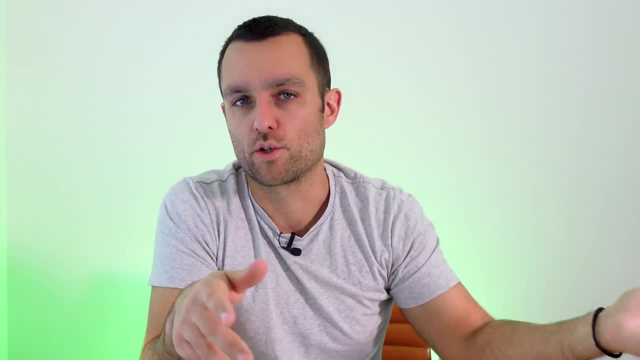 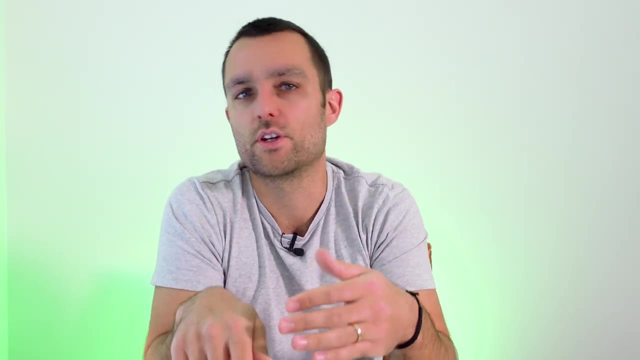 ambitious enough if you just kind of go a little bit above the benchmark, and that's it. For a lot of people they might be able to go way beyond the benchmarks. So you don't want to sell yourself short and just go. oh, the average is 50K and I'm making 60, so I'm doing great, I would say. 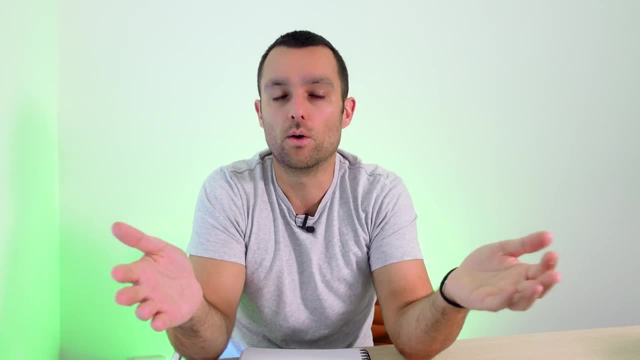 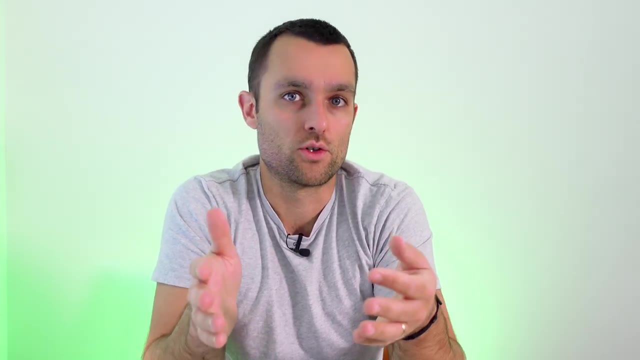 well, if you're capable of making 100 or 200 or 500 or more, then why not go for that? Take these numbers with a grain of salt. They are the official numbers, but it also shouldn't be something that you should use so seriously, And you should mainly focus on just trying to improve whatever you're. doing: If you're at 10K, go to 20.. If you're at 20, try to go to 40, and so on. So yeah, with that said, we'll go through the different ages. So 17 years and under is $199 per week And that works. 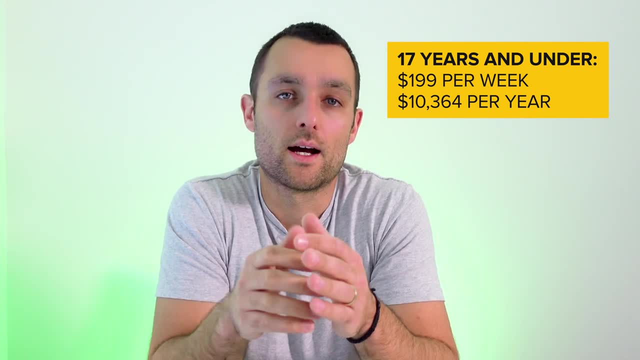 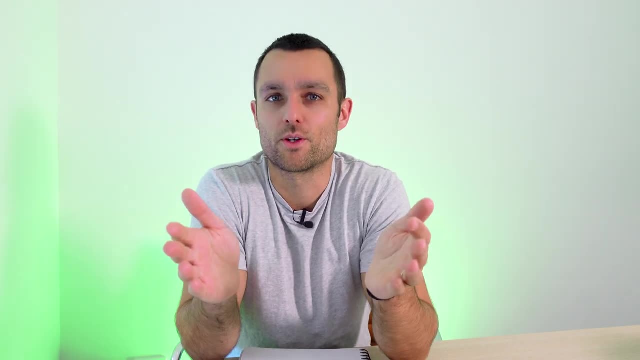 out to be about $10,364 spread out annually And, to be honest, this feels pretty low. I know that when I was 17, when I was 14, I was working at McDonald's and I was still at McDonald's when I was 17.. So to be making 10,000 a year it does seem a little bit low, to be honest, but I guess everybody Next up is 18 to 20 years with a weekly average income of $567.. And that works. out to roughly be about $29,500. when you spread it annually Now for 21 to 24 years old, the weekly average was $877, which works out to be about $45,500.. Once we get to the 25 to 34 year age, 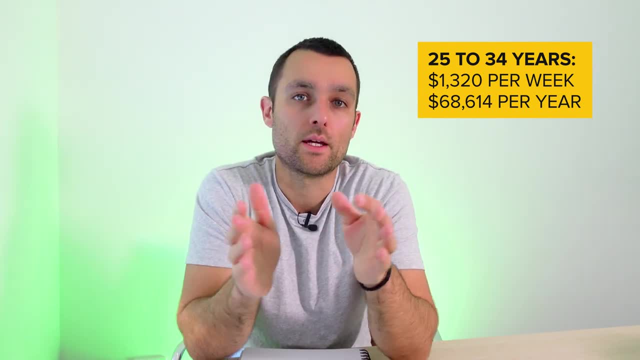 range. it does start to jump up a little bit, with the weekly earnings to be $1,320 and the annual earnings ending up at $1,000. So that's a little bit of a jump up. And then we've got the weekly. 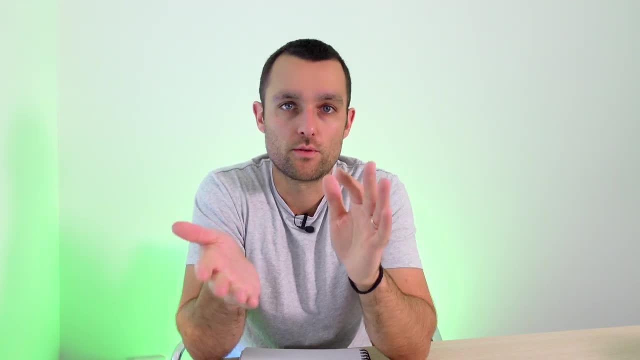 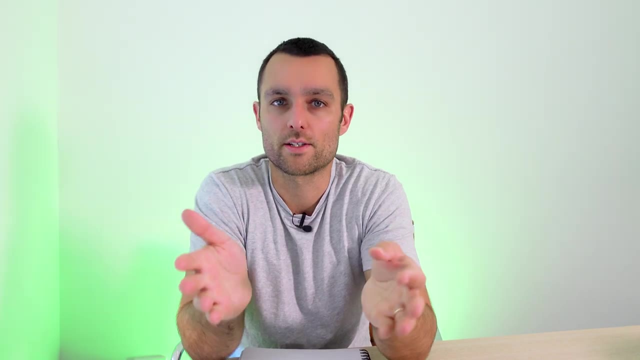 average being $68,600.. As we get into our 30s and 40s and 50s, obviously this is when earning potential starts to really surge For a lot of people. the classic phrase that I was taught was: first you learn, then you earn and then you return, obviously by giving back to the next. 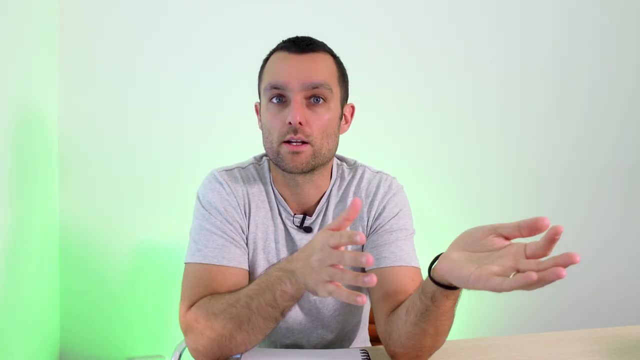 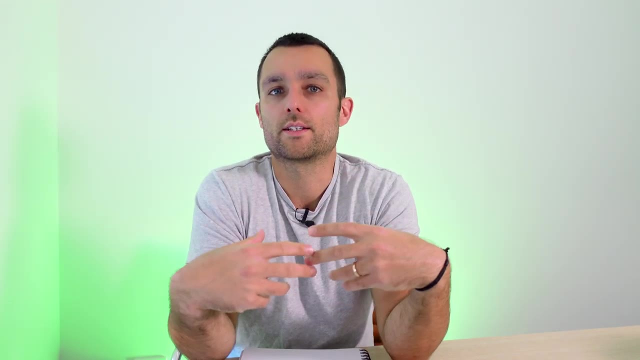 generation, And this is very, very true in the stats as well. You spend a lot of your teens and 20s and that sort of stuff learning And then, as you progress through your 30s, you really start to utilize those skills to start earning more. You've got a lot more experience by that point. So 35 to 44, it's $1,623 per week, which works out to be an annualized amount of $84,000.. Then we've got 45 to 54,, which is around $1,700 per week, And this is actually where it peaks in.